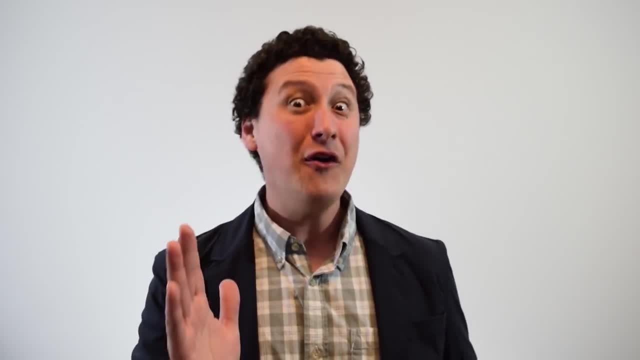 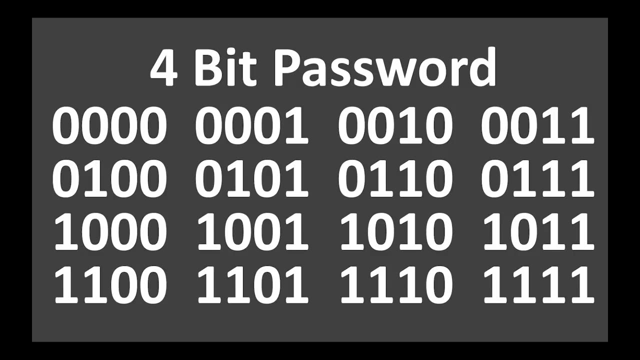 great, but what does this have to do with computers? Well, now is where the fun begins. Let's go back to those four bits. Let's say that I am trying to crack a password. The password I'm trying to crack is one of these numbers, but I don't know which one, So I've devised a machine to try them. 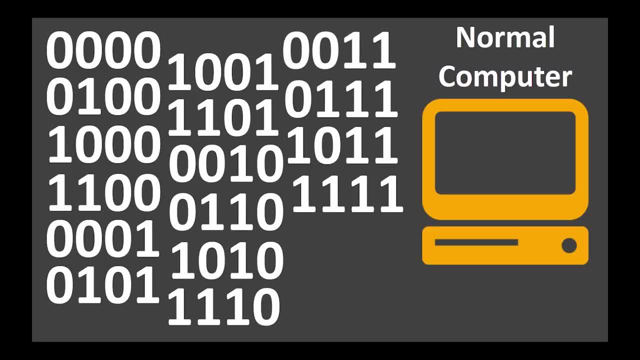 all, This is a normal computer. I take one number, I put it in my machine and then I put it in my machine. If it's wrong it gives me an x, But if it's right, if the password is right, then yay, I've. 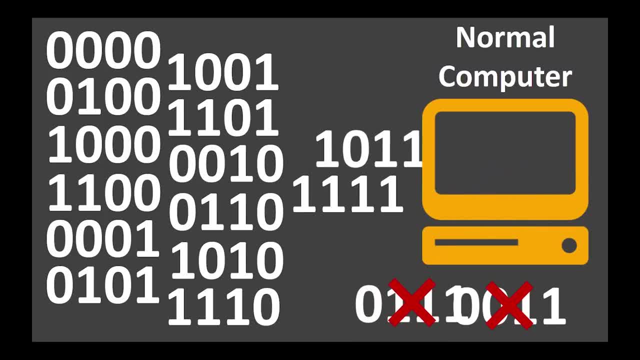 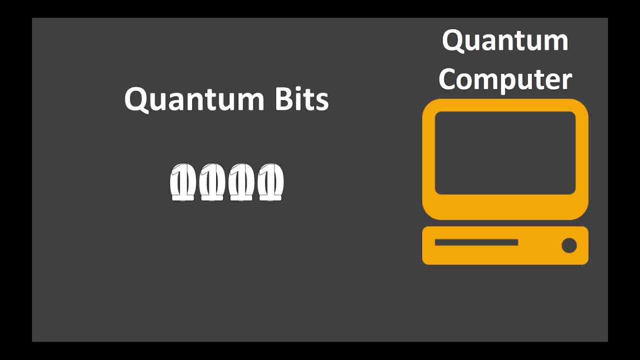 got the right number. So a normal computer will try each and every one of these individually until it finds the right answer. Now what if we use a quantum computer? So instead of putting in these four regular bits, we put in four quantum bits. Now remember, each bit is both a 0 and a 1.. 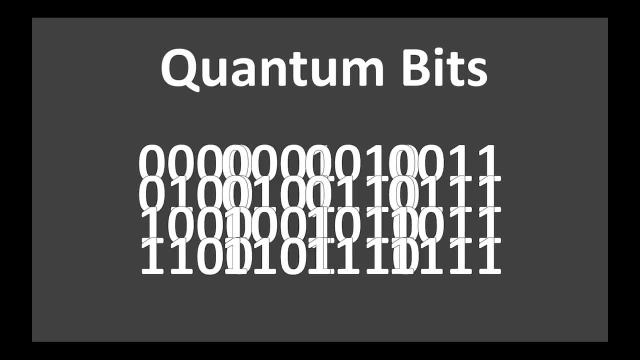 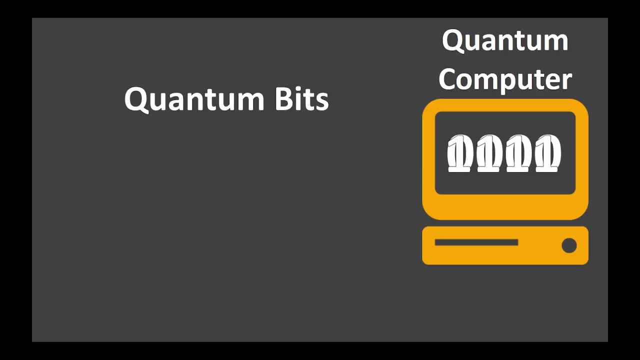 That means these quantum bits are all the numbers all at the same time. So when I put the quantum bits into my machine to find the right password, what comes out the other end? Well, turns out, the machine is saying that I'm both right and wrong, because I gave it both right and wrong answers at the same time. 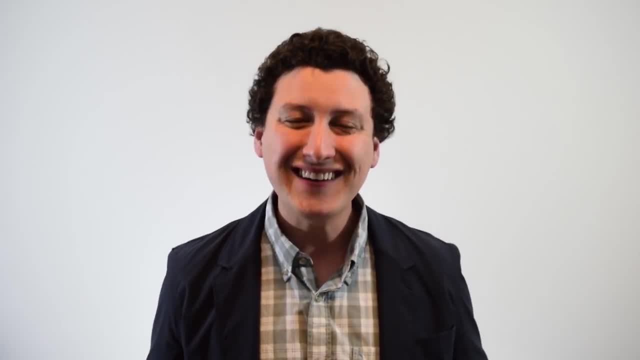 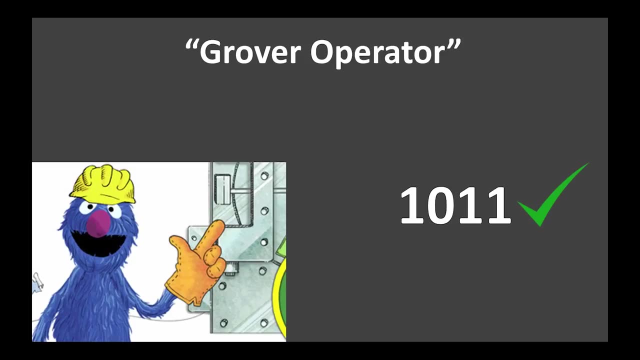 I still want to know what the correct password is. Well, there's a technique called a Grover operator. okay, this is actually a real thing where you can sweep away all the wrong answers and what you're left behind will be the right answer. So what I'm going to do is I'm going to 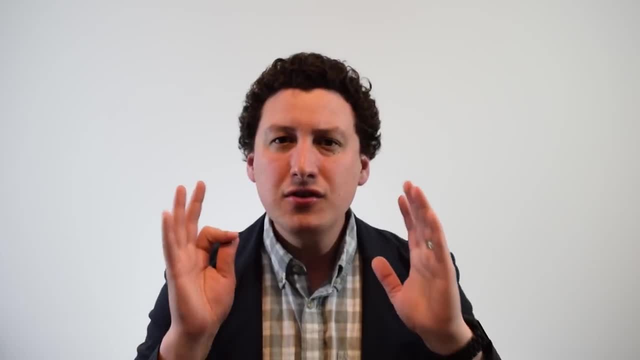 move the mouse over to the wrong computer. and I'm going to move the mouse to the left. So one of the problem: if you don't know where to where to find the answer, you'll need to figure out how to find the answer. Okay, so, for example, the three numbers: 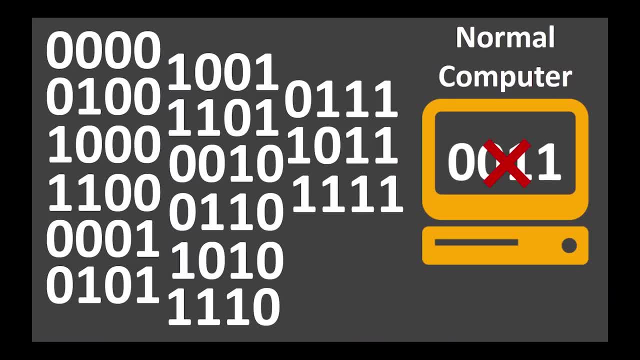 one is 0 and one is 8.. So I'm just gonna move my mouse to the right and what I did was I could use a computer, and I could use a computer to try each and every one of these- and that's the beauty of quantum computing- Instead of trying each and every value like a. 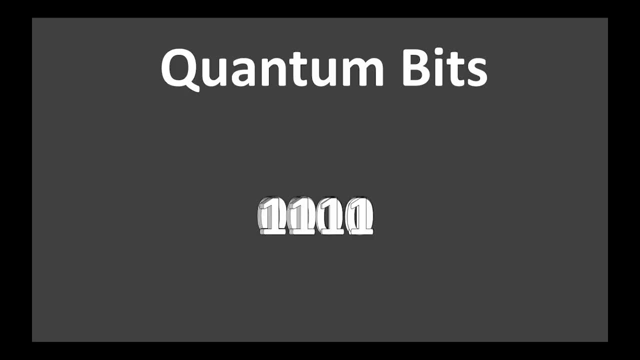 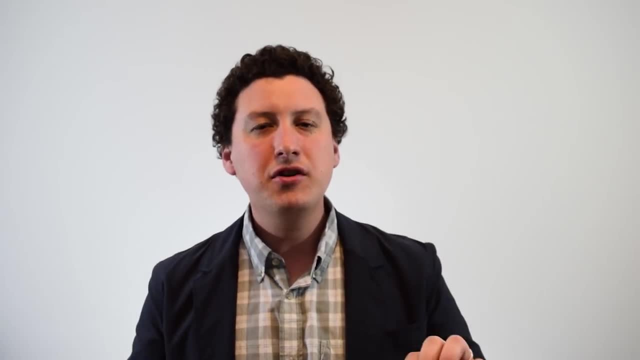 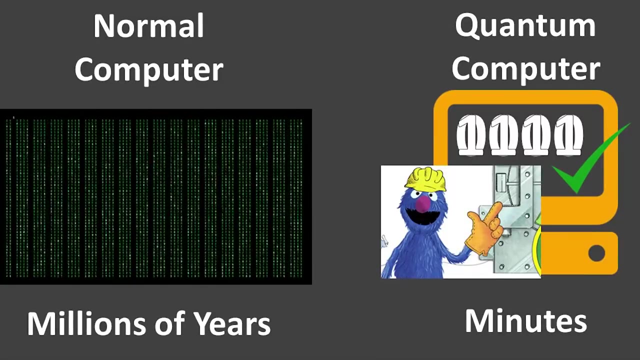 normal computer would. a quantum computer tries them all at the same time. But in real life, high security, encryption, those would take a regular computer millions of years- In fact I heard some people say the age of the universe- to try and crack these codes. That's how secure. 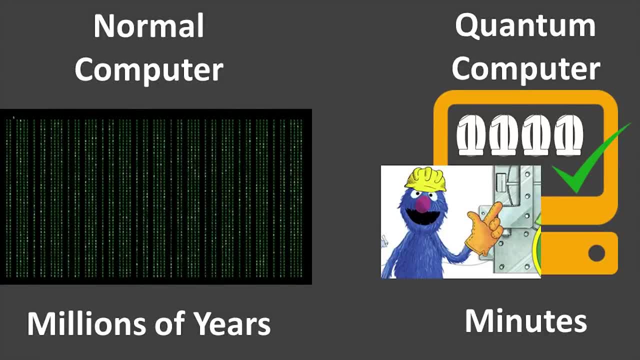 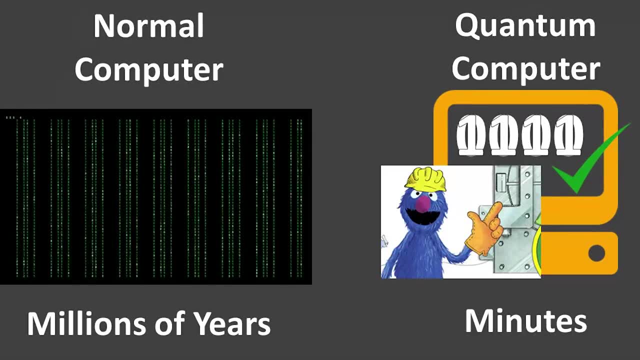 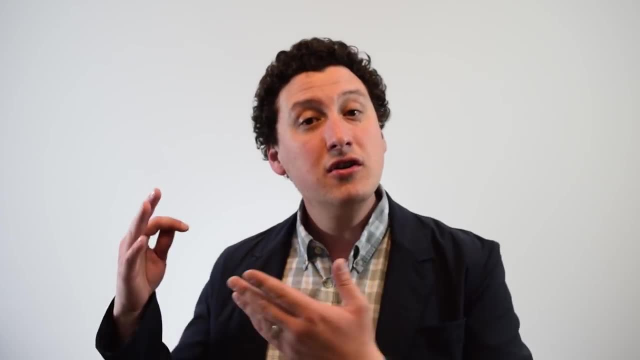 they are, But with a quantum computer you can try them all at the same time. Use the Grover operator to sweep away all the wrong answers, and what you're left with is the right answer. So instead of taking millions of years with a regular computer, you can do it in seconds with a quantum. 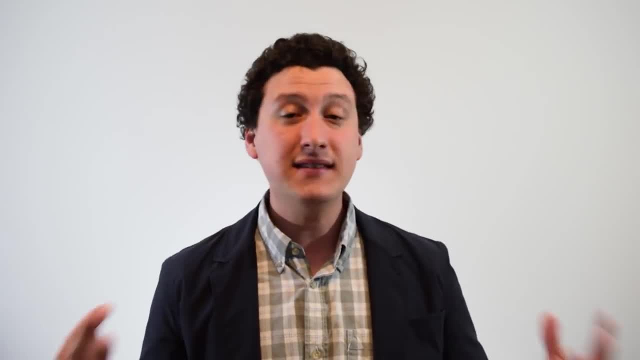 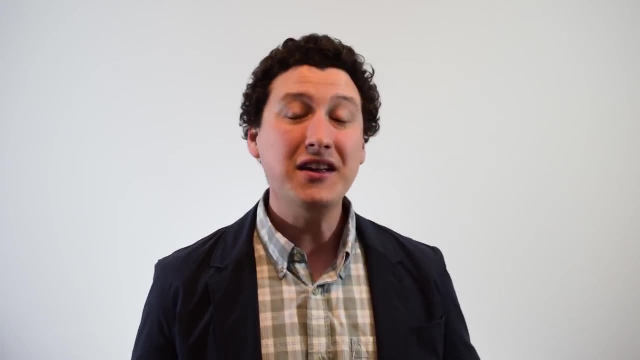 computer. Now, what are some other things you can do with a quantum computer? Well, let's take something we're really familiar with. What about a point Distances between two points? What Google Maps does, what regular maps do, is they look at all the different possible paths between two points. 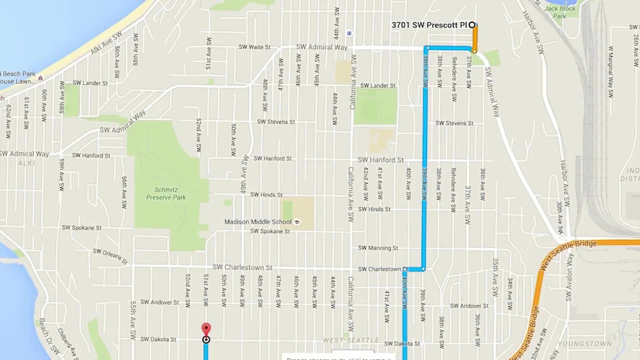 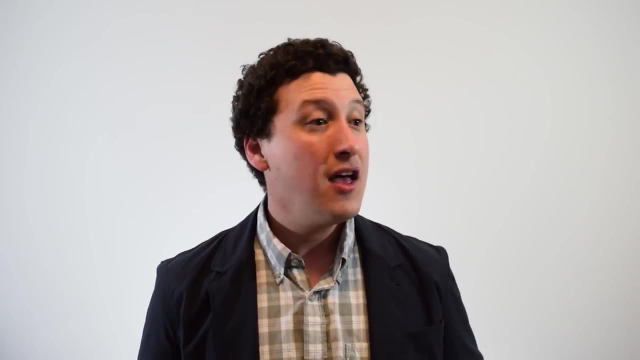 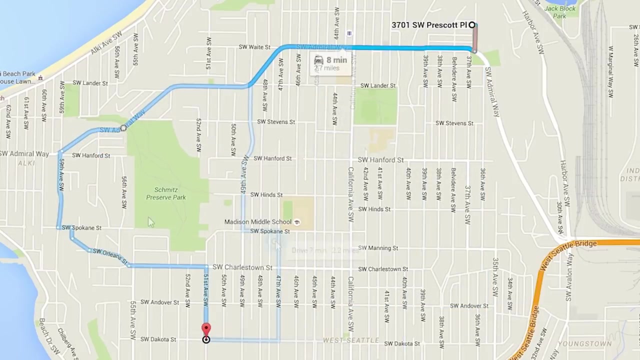 They try them one at a time and figure out which is the fastest one, which is the shortest distance, which is the optimal one. and that takes a long time, That takes a lot of computing. With a quantum computer you can try every possible path between two points all at the same time. 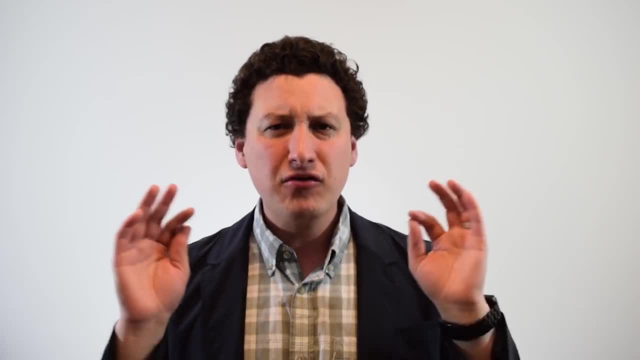 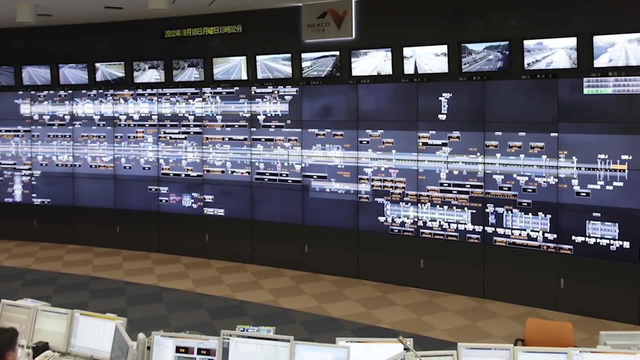 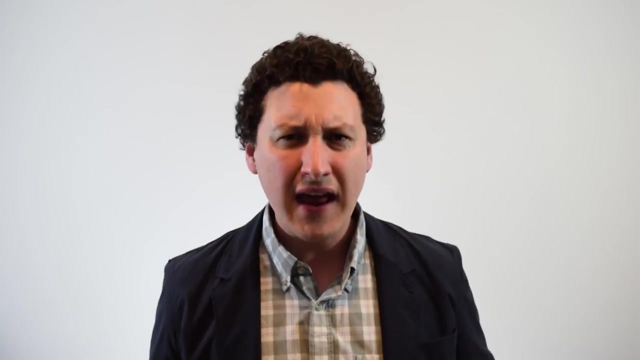 And pick the best one. Okay, this is huge because the rise of self-driving cars is coming, And imagine having a master system, a master quantum computer, managing the entire system, optimizing every vehicle that's out there on the road, figuring out the best alternative routes to avoid. 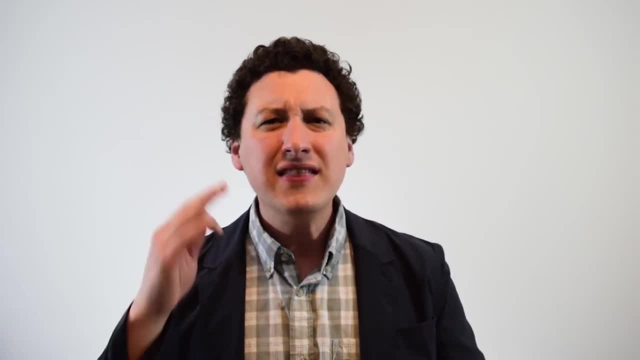 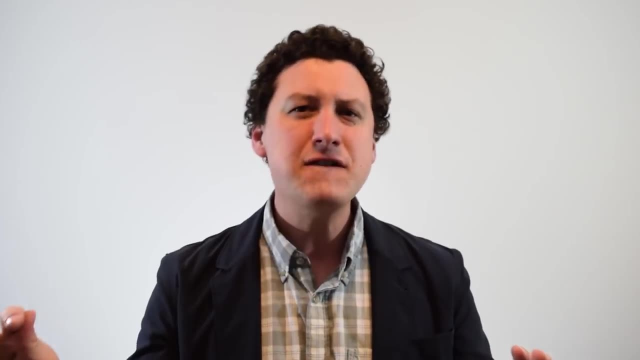 hazards and avoid accidents and to and figuring out when the lights should turn green and red, And suddenly you have the best possible commute, because it's literally tried everything in the universe and has found the best way to do it. So let's take a look at a quantum computer and pick the best one. 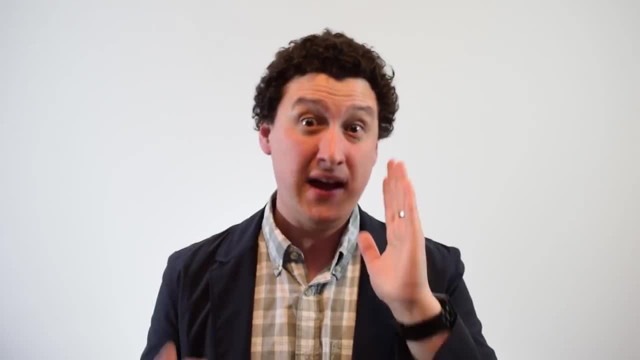 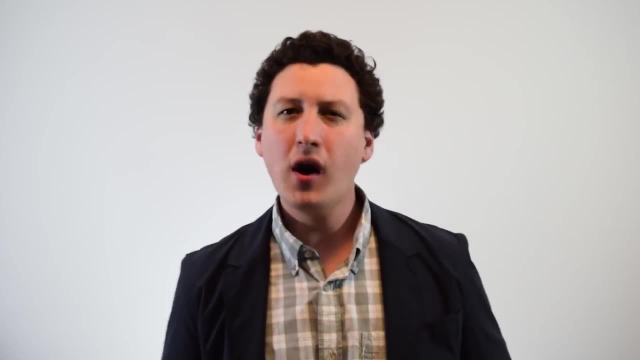 The one solution that is the best that works. Okay, that's a quantum computer. Regular computers could never do that. Okay, what about artificial intelligence? What if we gave a quantum computer the ability to reprogram itself? Well, computers don't really know the best way to reprogram. themselves. A normal computer would would have to do trial and error and see what works and what doesn't, what makes itself better and what doesn't. But a quantum computer can try every single possible program And find the best one. It could try every single possible circuit design and make itself the best. 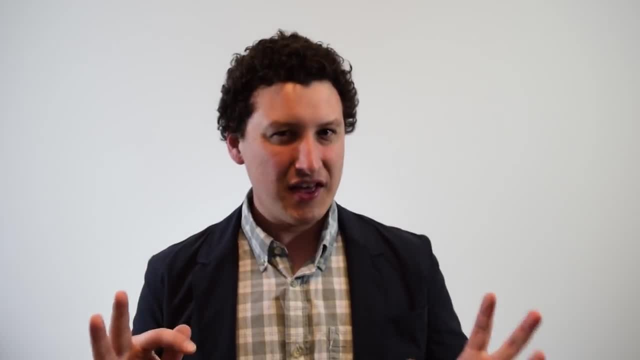 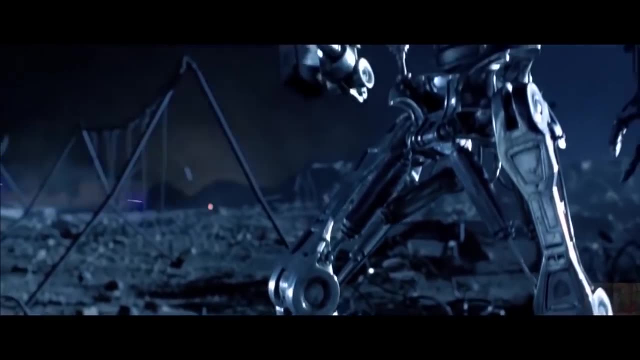 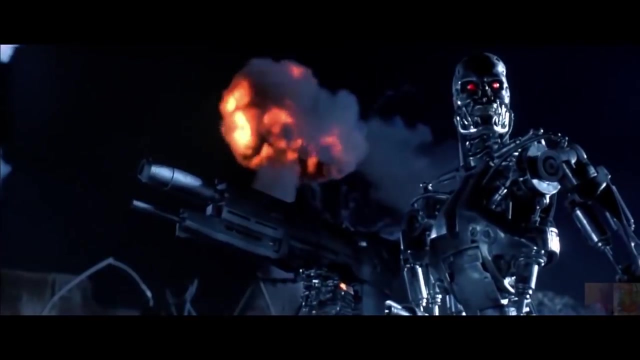 Okay, and that's kind of scary, because in an instant the quantum computer could figure out how to reprogram itself and remake itself into the best possible artificial intelligence ever, And if that doesn't blow your mind, I don't know what will. Okay, that was it. Hopefully this video was an aha. 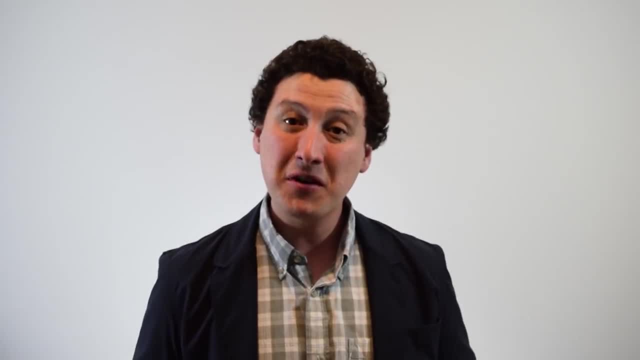 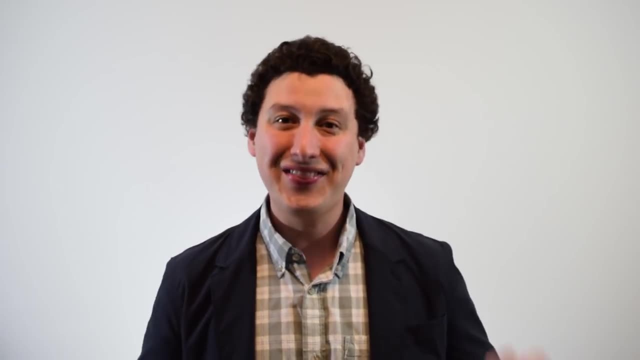 if you didn't already know, maybe now you understand how quantum computers work and what the implications are. If you found this video useful, feel free to like the video and do share this video, and thank you very much for watching.